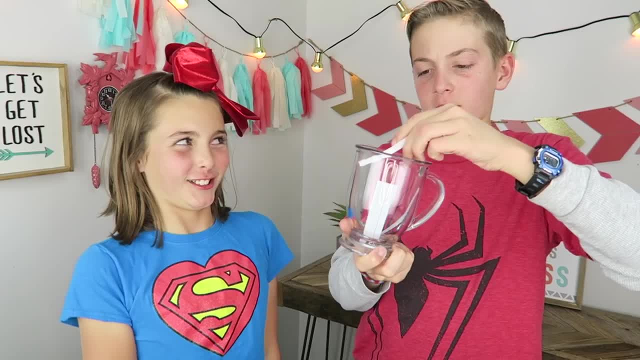 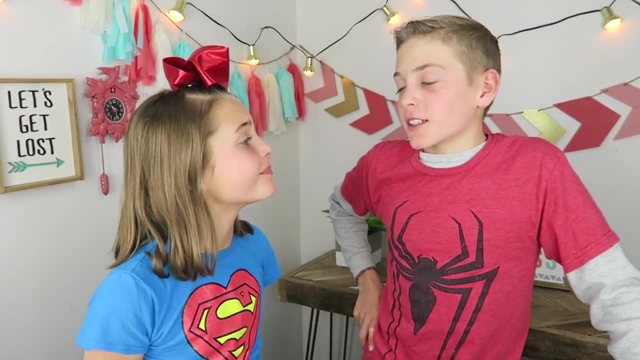 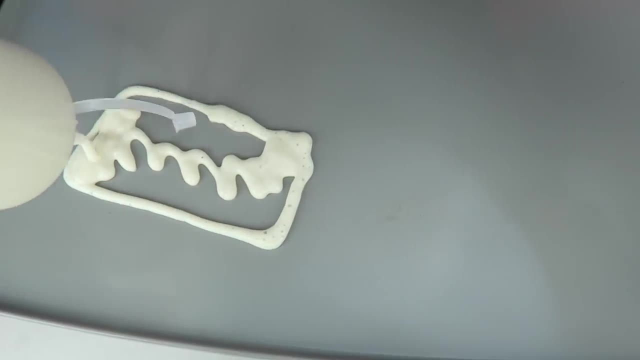 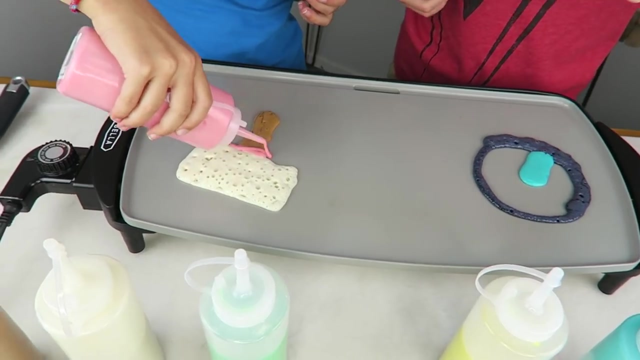 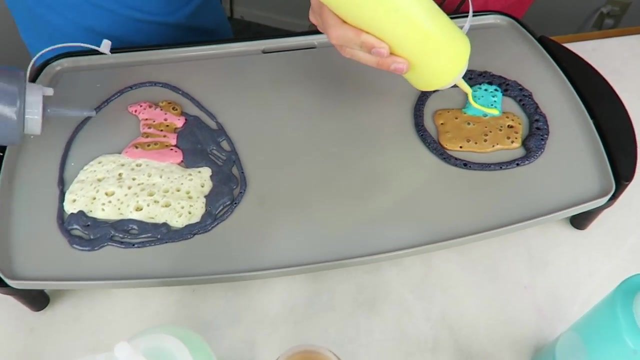 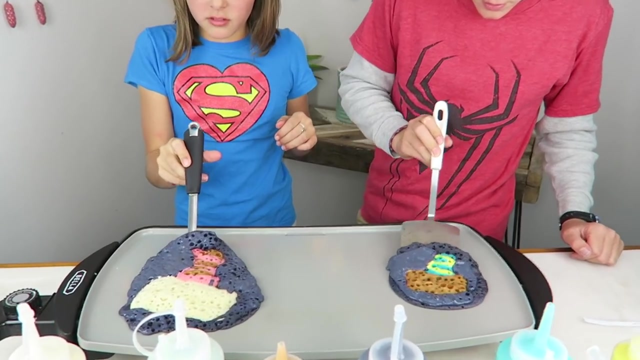 go first, Corbin, I'm going to now. Okay, Thor, Oh, dang it, Thor. So I think his symbol is his hammer with like a circle thing around it. Okay, Yeah, I have a big one. Oh wait what? Oh, no, no, don't break, Don't break. yeah, look at that. 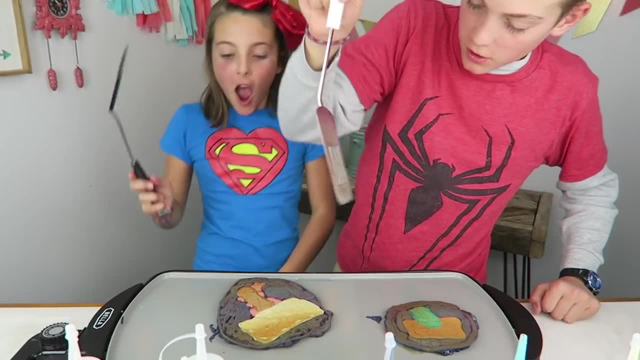 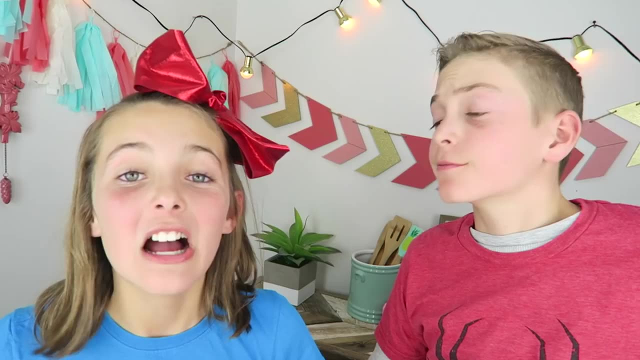 Can you help me flip mine Set go. Oh yeah, Look at that. Bad Baby, Bad Baby. Okay, guys, time for you to vote. Who's is better, Mine or Corbin's? Mine, No, it's mine. 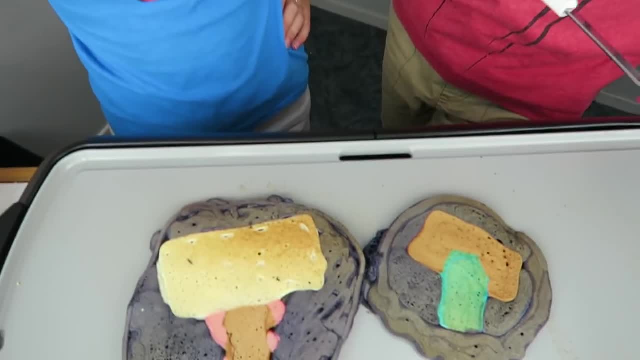 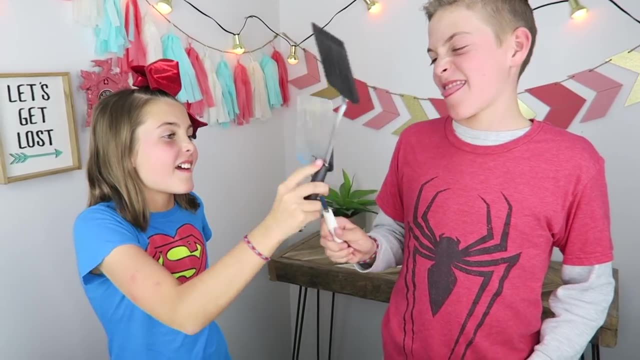 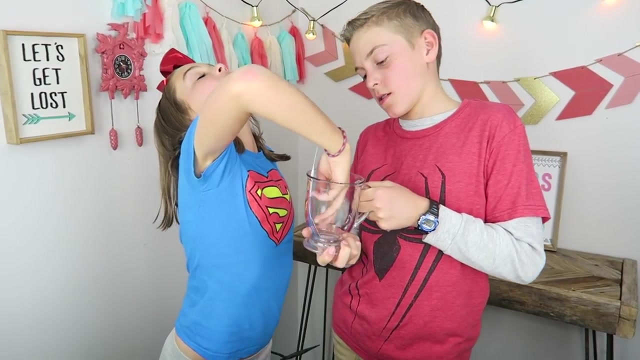 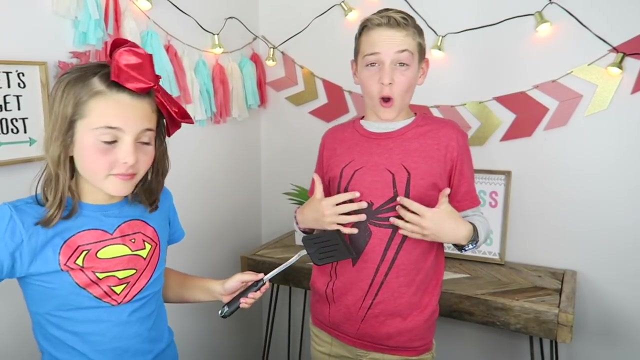 No, I mean obviously mine. Yeah, You hit it Honestly, mine. Okay, on to the next one: High five, I got it So creepy, Your turn. I got Puddlemon. Okay, I'm Spiderman, so I totally got this, you guys. 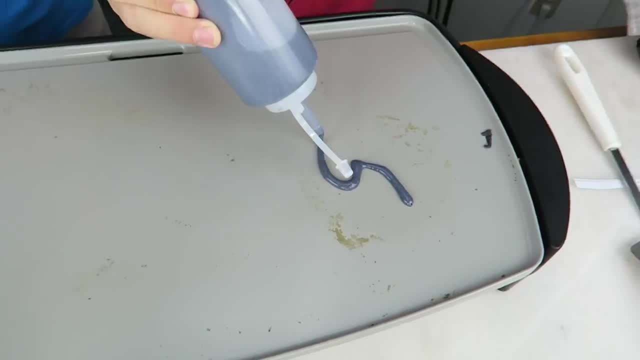 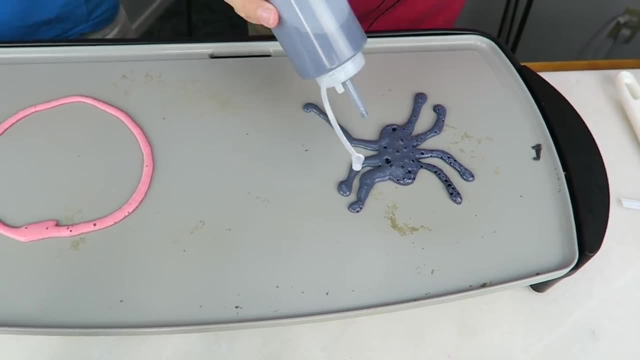 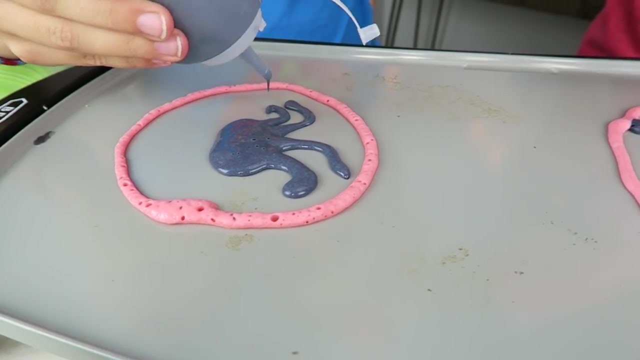 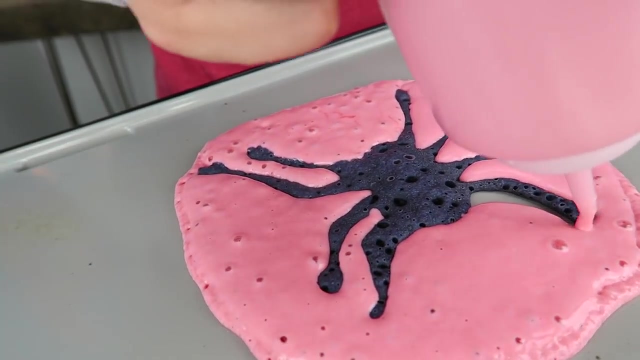 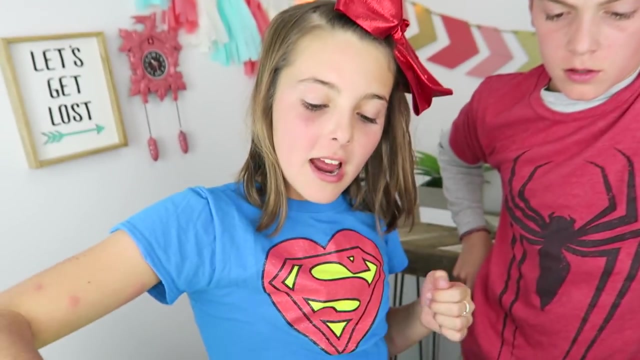 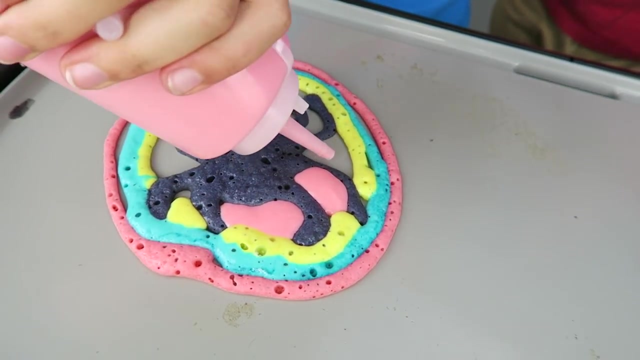 No, but I can look at your shirt. I totally got this. I got I'm gonna make mine like a rainbow in the background because, I mean, spiders are very colorful in their own way. I just like these pretty colors, so I'm gonna do them. 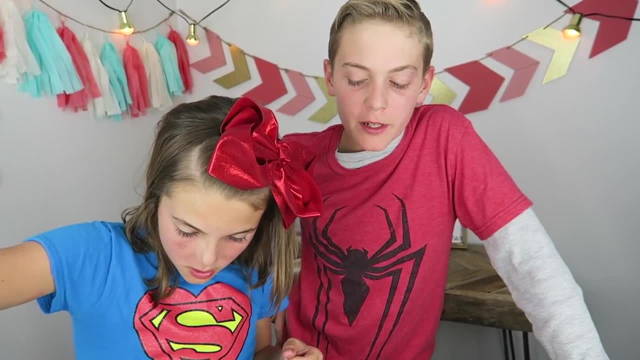 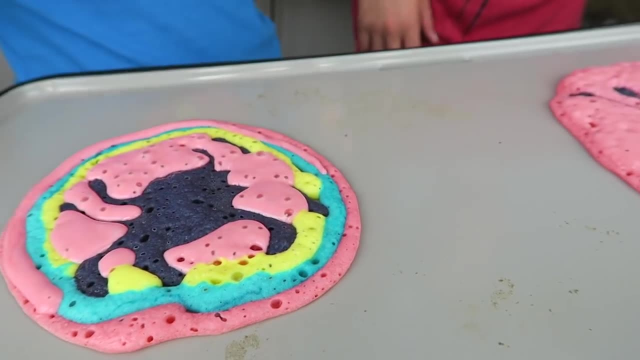 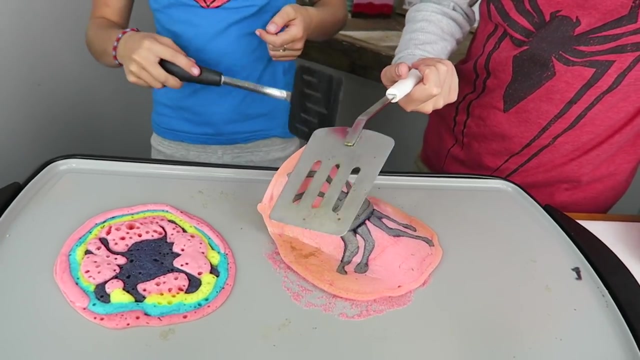 because? But Spiderman isn't supposed to be pretty, He's supposed to strike fear into the hearts of his enemies. Okay, And then just let it crackle. Oh, it's not going off. Oh, no, no, no, no. 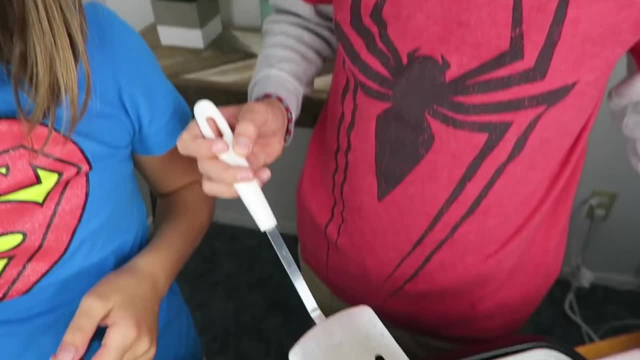 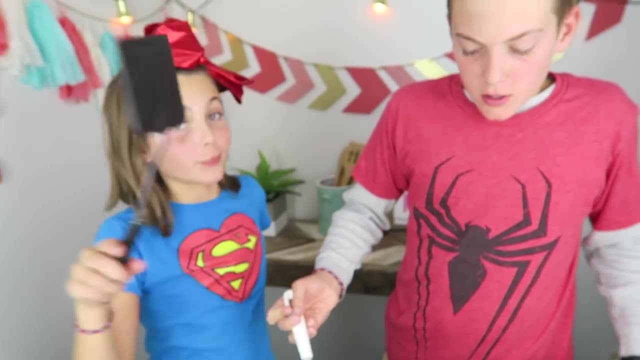 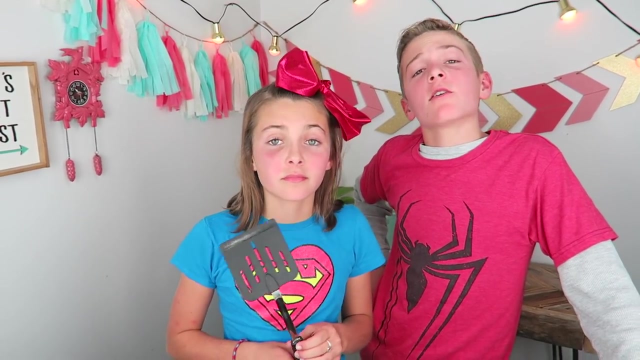 No, No, That's why you make it small, so, So it doesn't break. No, Oh yeah, look at that. Boom. Spiderman round is over. Now it's time to comment on this round. Who do you think won? 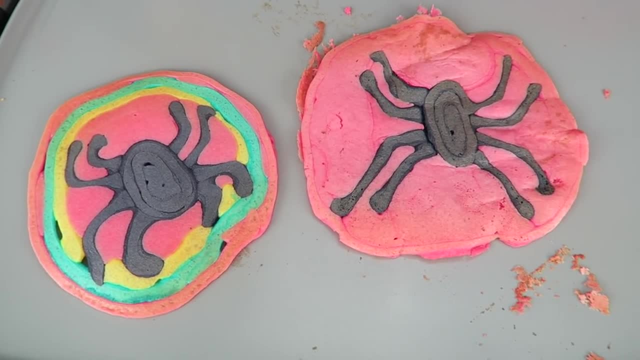 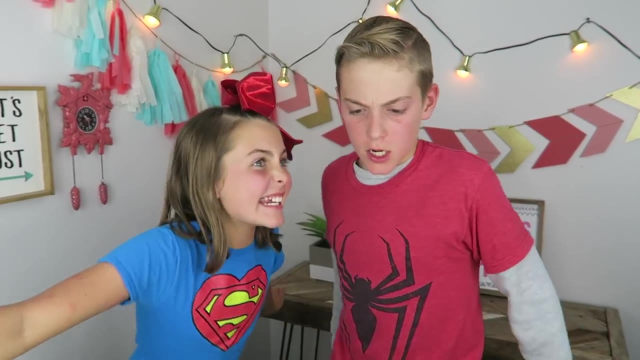 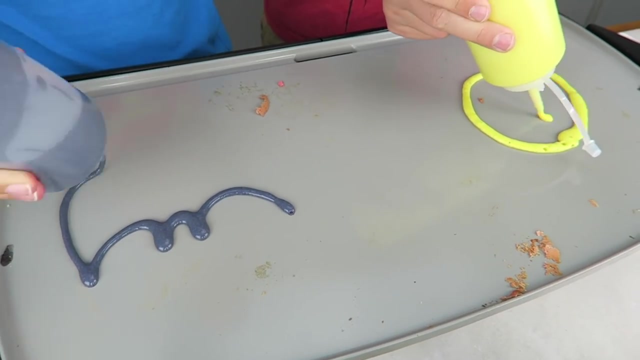 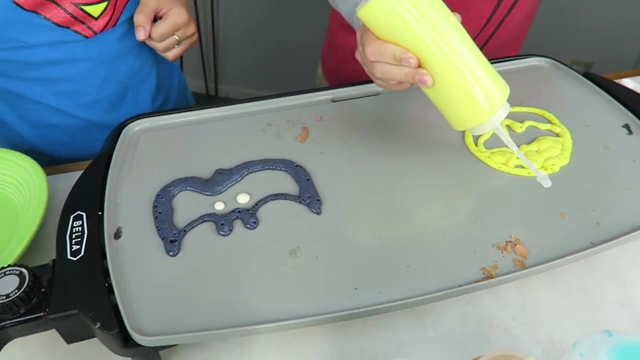 Me, of course Me. It's obviously me. Spiderman, Me, Correct, Batman, Batman. I'm gonna start with yellow. I'm gonna do black. Okay, It's starting to look like a seagull, Or maybe like an airplane. 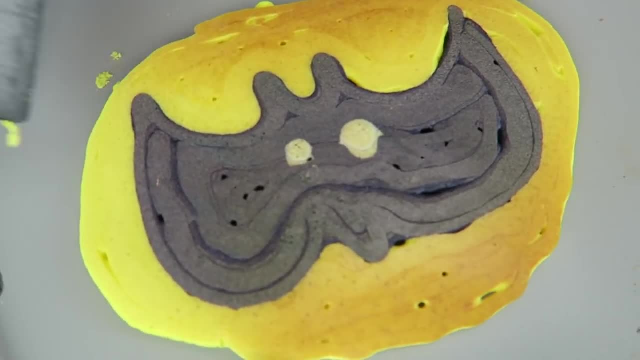 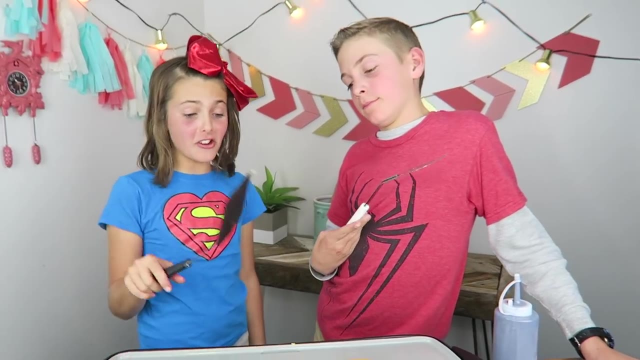 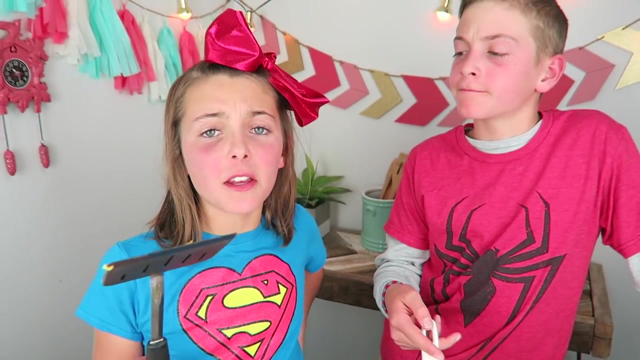 Yeah, Oh yeah. look at that. No, Put eyes on mine. It looks like a big mustache with eyes. Yours looks like a black blob, That's true. Okay, guys, time for you to vote. Who won? me or Corban? 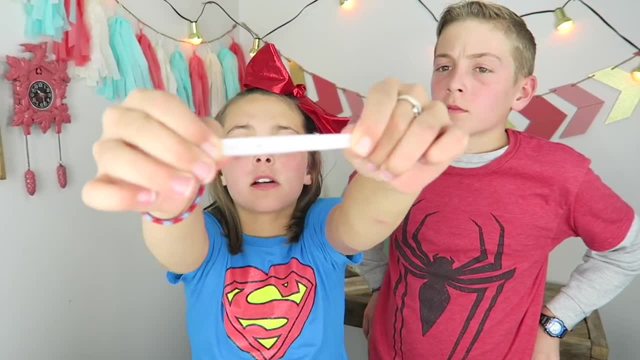 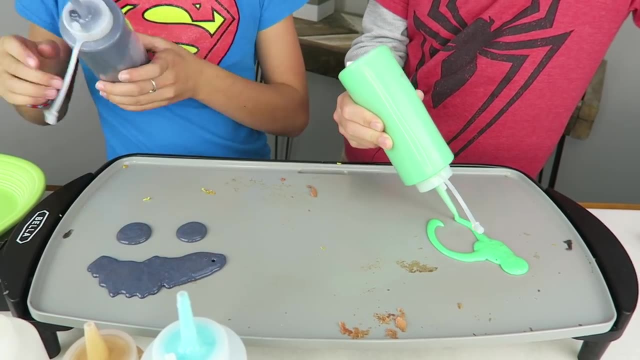 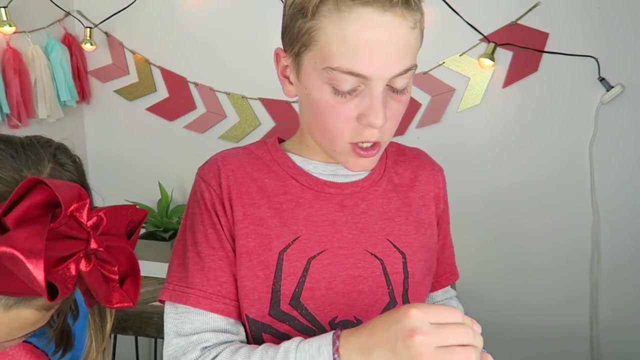 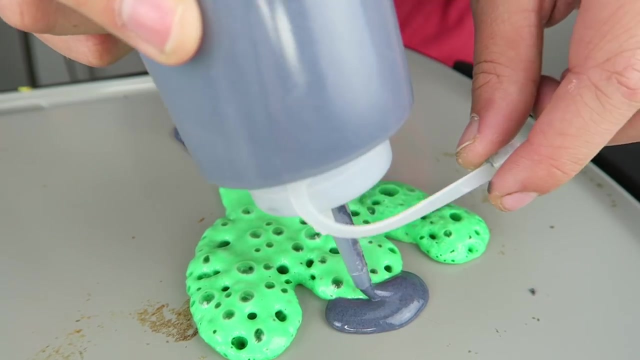 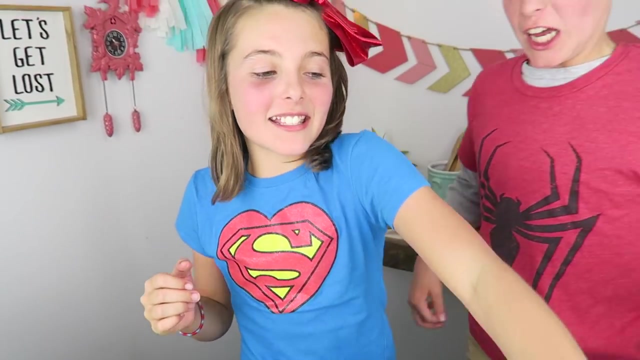 Let's see who I get. I got Hulk. He's gonna be like flexing his giant muscles. Oh, I forgot his hair Right there. Okay, and I forgot his hair. Hulk is like a big green blob. I forgot, I forgot, I forgot his nose. 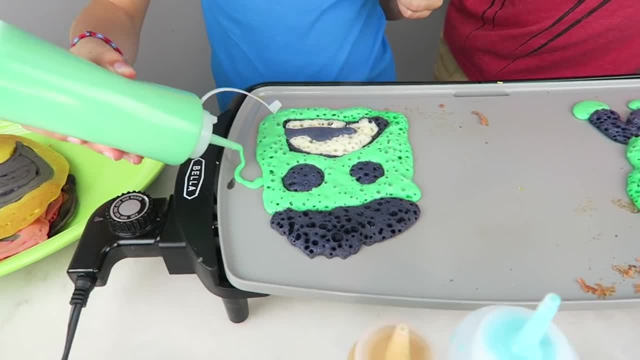 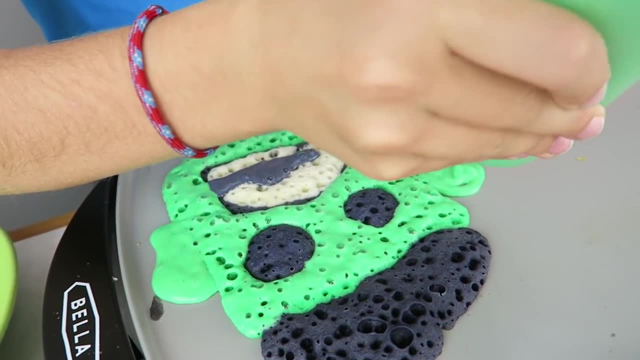 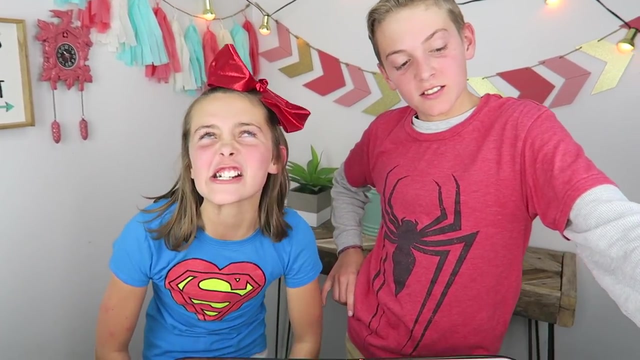 He's like grrrr, And, but don't worry, I won't forget his ears, His big green ears. That's hilarious. And then and then he's like going like a grrrr, grrrr, something like that. 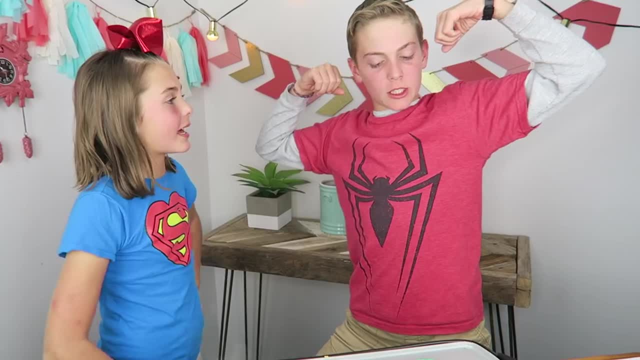 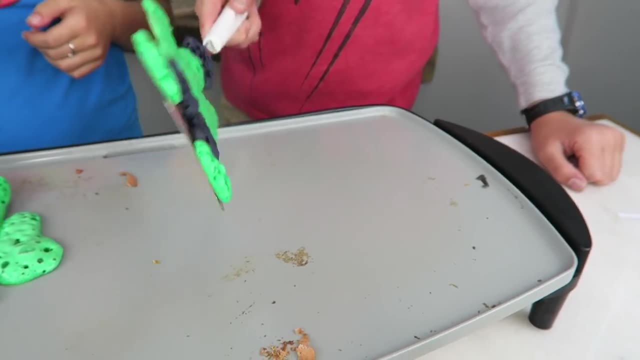 So for me he's just like going like this and he's like grrrr. No, he's like this bluh. He got his big pants and his belt on. that's why his waist is so tiny Flip. 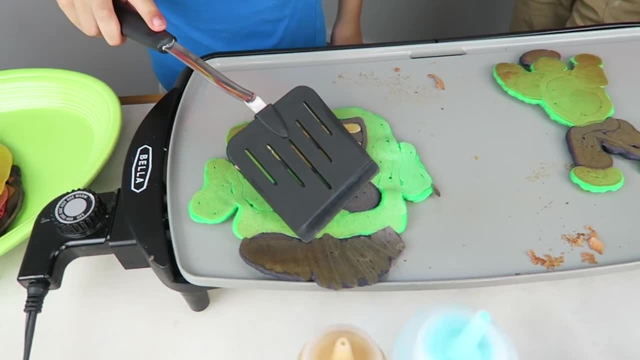 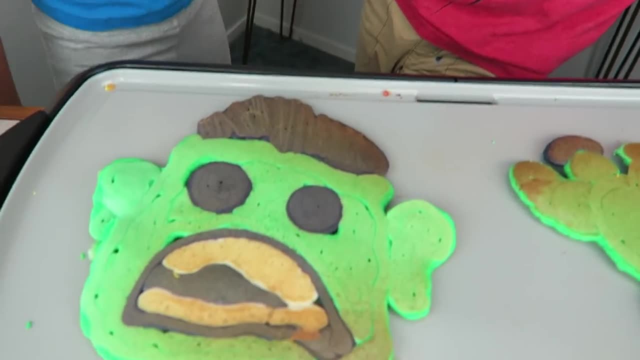 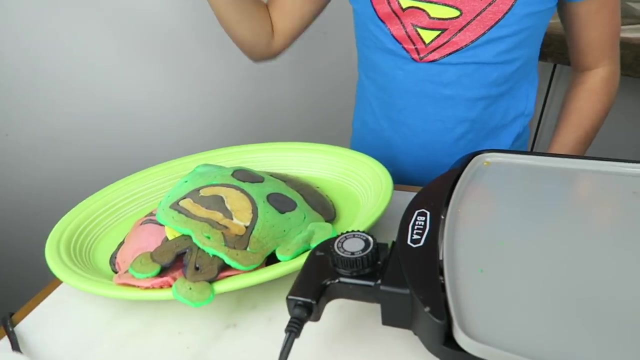 Yes, please, Yeah, Flip, oh yeah, Who do you think won me? or Ava? Hulk smash, Grrrr, And if you don't vote me, I'm gonna find you and Hulk smash Me too. All righty people. time for the next one. 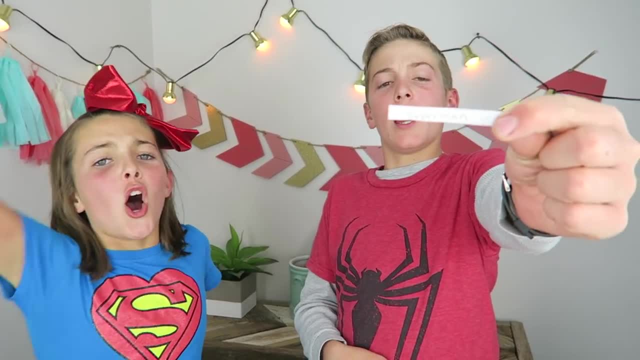 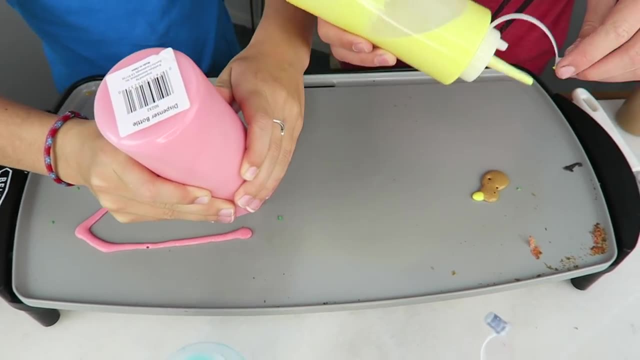 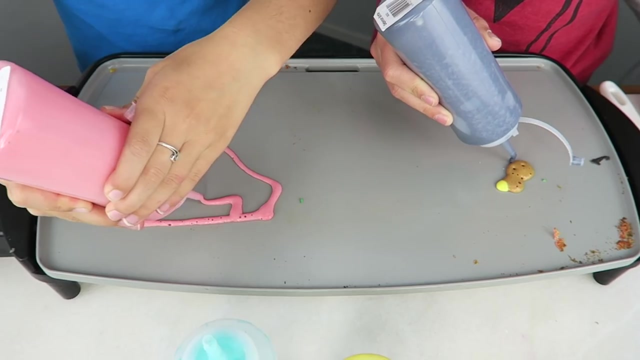 We are going to do Superman. Yeah, I'm gonna do pink, And it goes like that, and it goes like that. it goes like that, It's in wait, it's gonna be backwards. so This is so hard writing an S backwards. 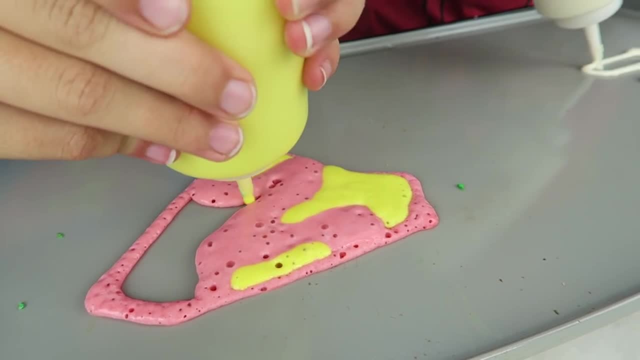 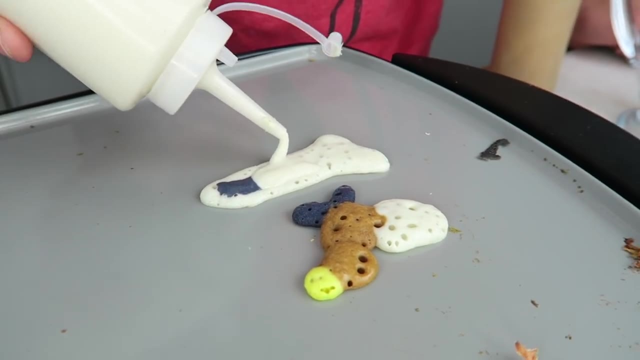 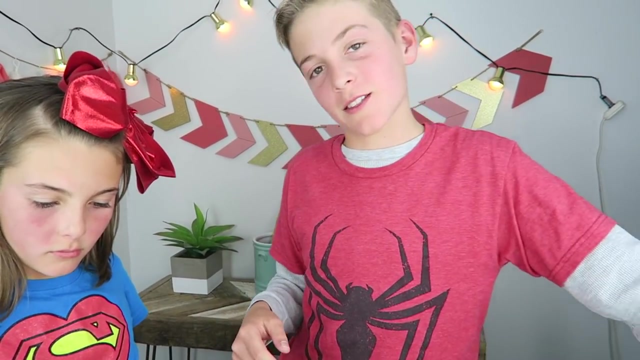 It looks like a Z. So what I'm trying to do right now is make a bird and a plane, just like in the saying: it's a bird, it's a plane, it's Superman, And then you have, like, the Superman symbol. 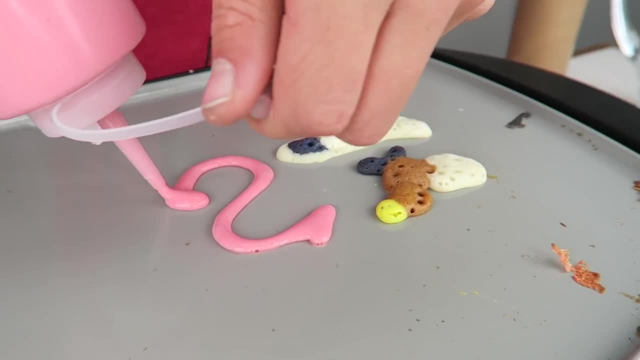 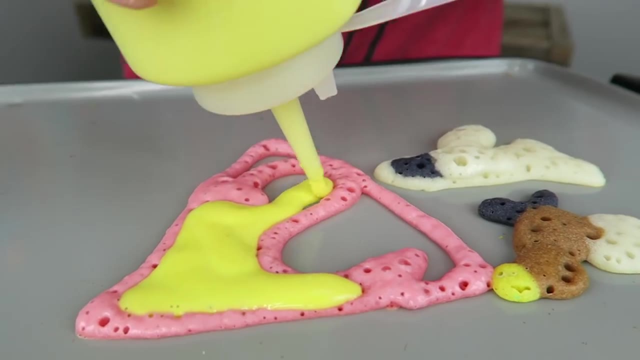 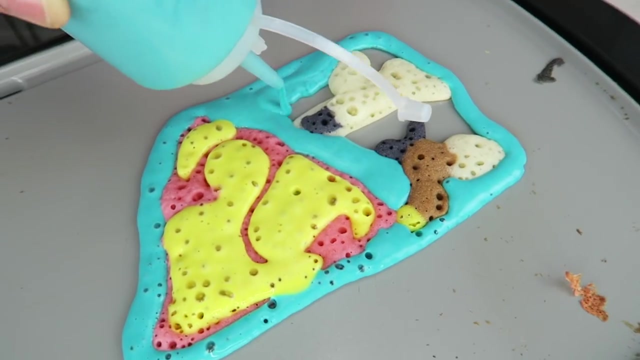 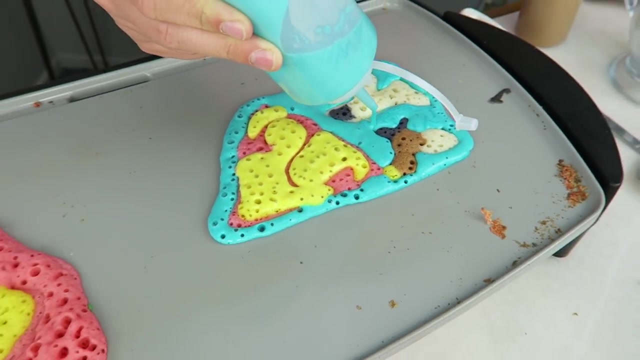 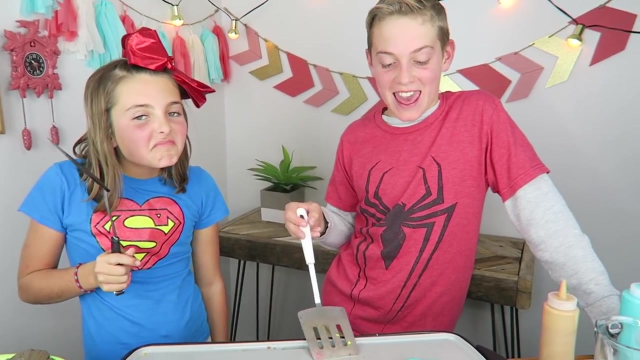 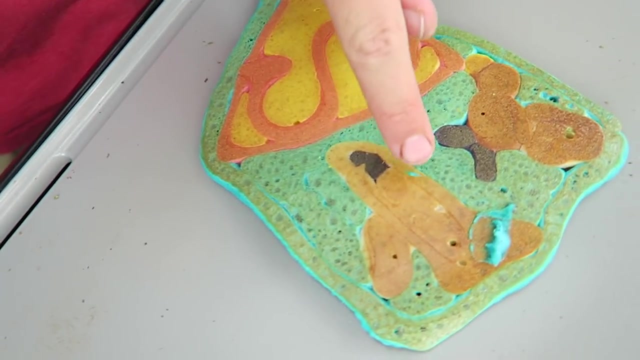 right next to it. it'll be awesome. Okay, in the final, Huh, Guess what? It's a bird, It's a plane, but no, it's Superman. Yeah, drink, Drink, Drink, Drink, Drink, Drink. 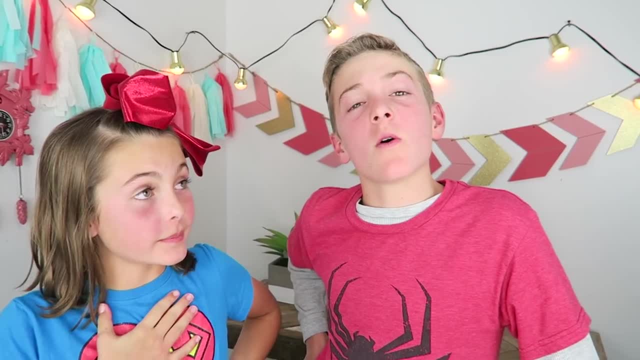 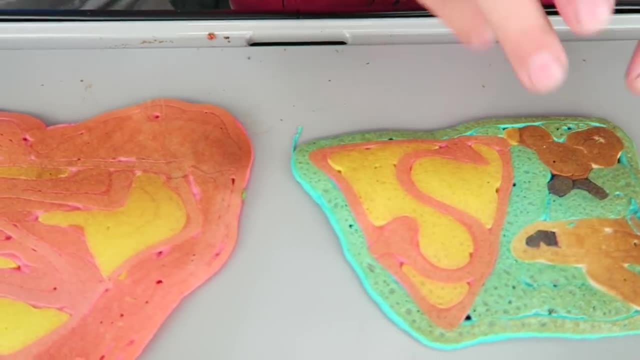 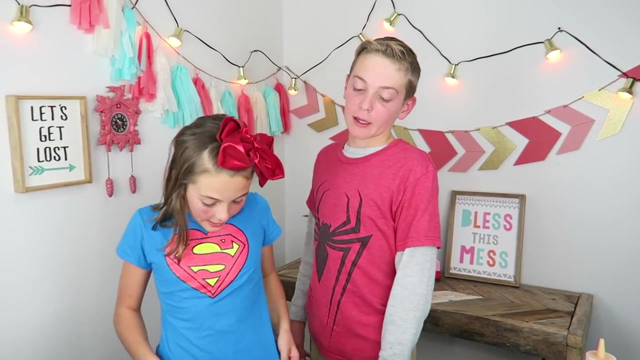 Drink. who do you think won on superman round me or ava me? it's obviously me, because i got like the bird it's playing superman sort of thing going on. that's just like a blob. how dare you? it's a big plank. hey, i was just copying off my shirt. it's a plank blob. 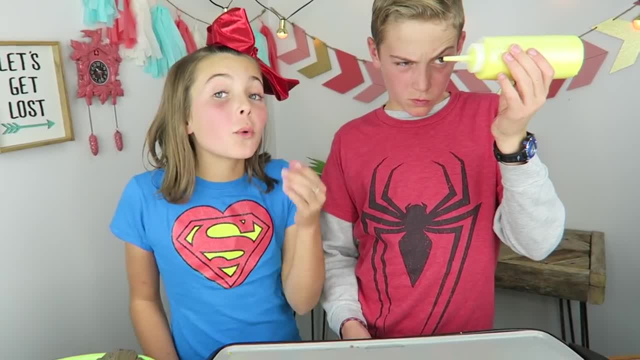 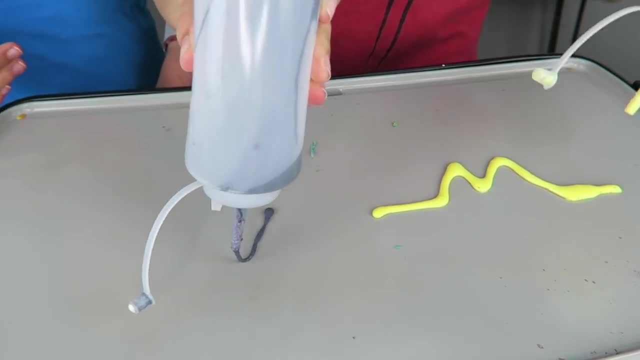 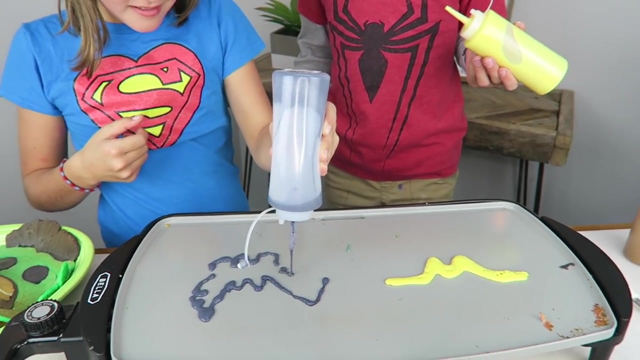 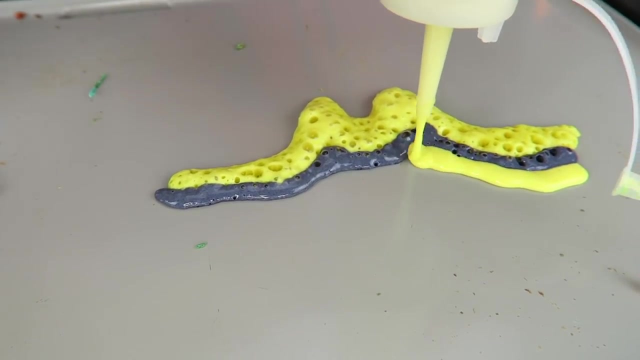 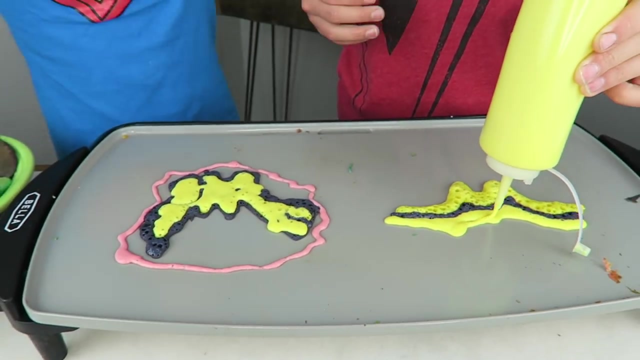 okay, last one. we're gonna do wonder woman, except we're gonna use our left hand, gonna be. this is so bad. can i see that, ava, it's a lot better than mine. i'm not very good with my left hand, so, yeah, we're gonna quit being me. 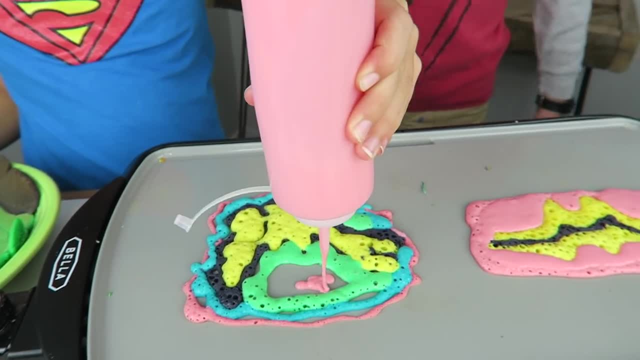 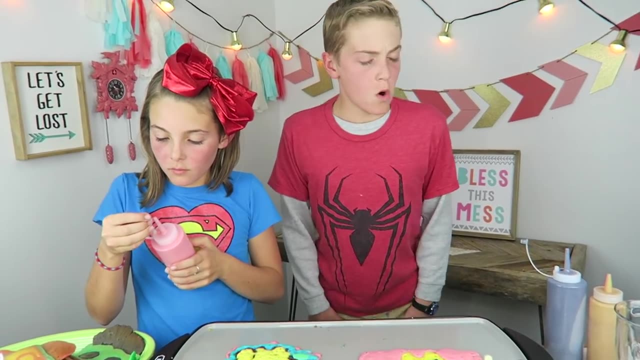 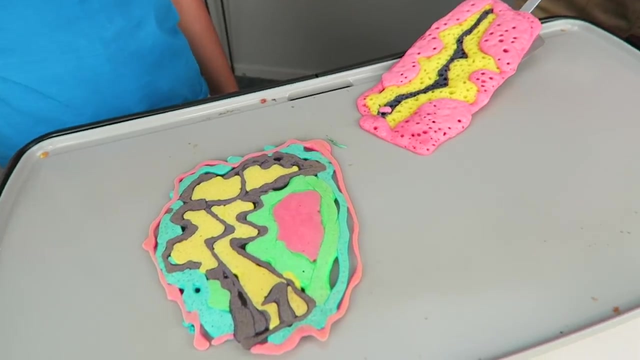 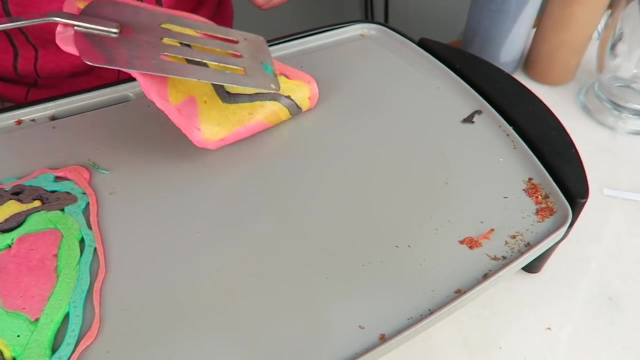 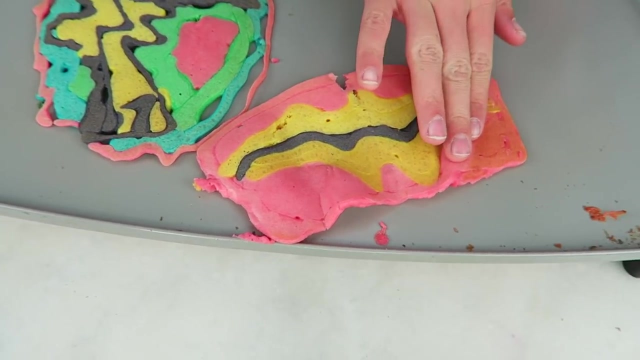 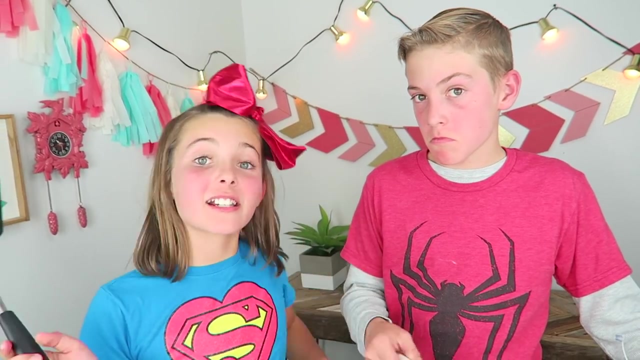 there you go, ava. all right, i think i got this one. i got this one. oh, i got this. okay, time for the great reveal. you ready? no, you failed, you failed. you failed. there we go. okay, guys, time to vote. who's is better, mine or corbin's comment down below.